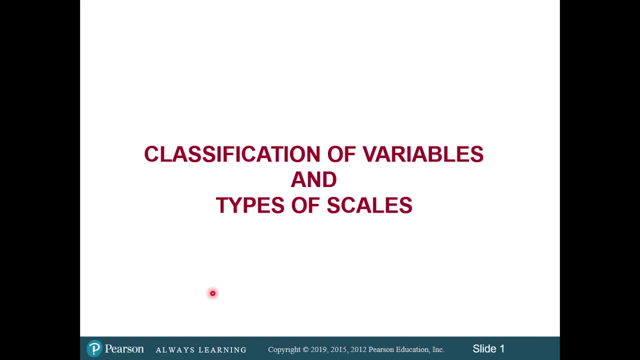 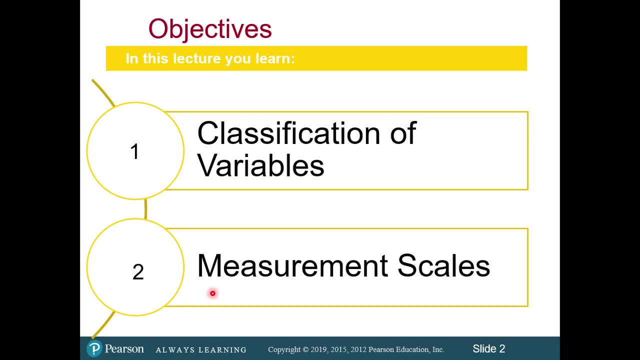 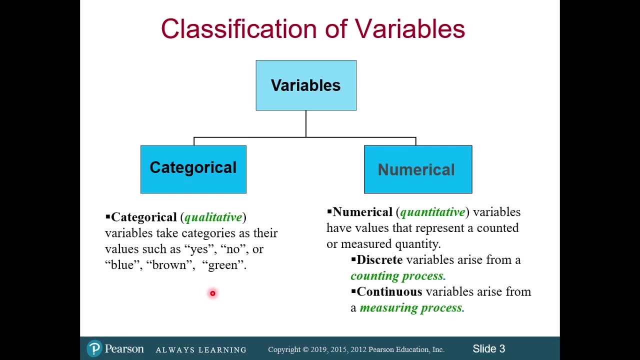 In quantitative research it's very important to have basic understanding of the classification of variables and types of scales. So in this short video I will be covering these two important points. Variables are generally classified in two forms: One is categorical, other is numerical. 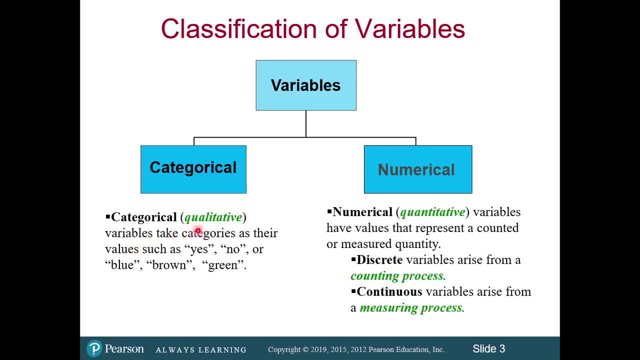 Categorical, that are qualitative variables. they take categories as their values, such as yes, no or blue, brown, green. So these are categories and taken as values. Yes is one category, no is another category. This can be changed. No can come first. yes can go second. 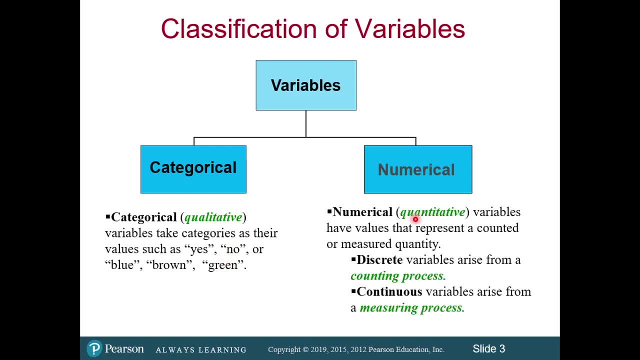 It doesn't matter. Numerical variables are those especially. these are quantitative in nature and have values that represent a counted and or measured quantity. Remember, most important point here is counted or measured. When it comes to counted, these are discrete variables. 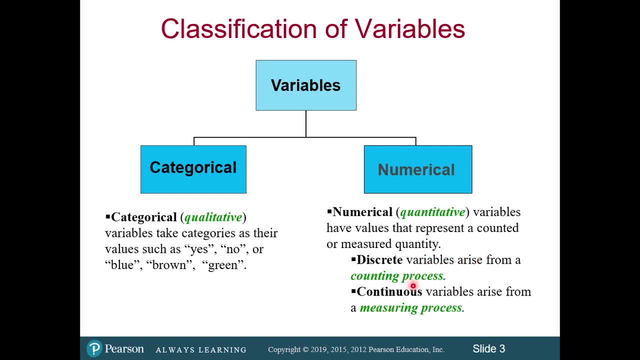 Discrete variables arise from the counting process, But Continuous variables arise from the measuring process. So that's why all the numerical variables, either they will have counted or measured quantity. If counted, these are discrete. If measured, these are continuous. 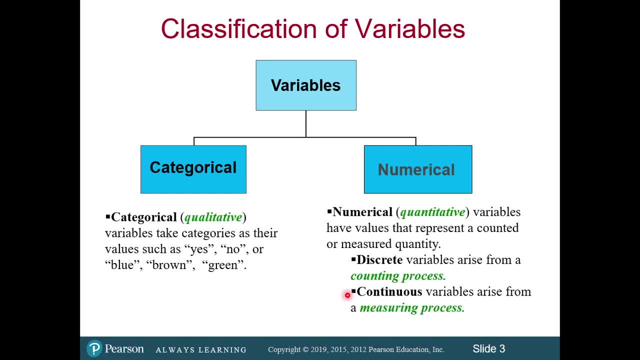 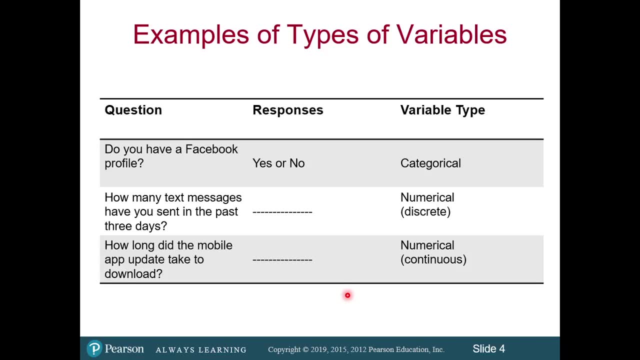 Let's understand what is counted and what are the examples of counted versus measured quantity. Let's say The question is: do you have a Facebook profile? If that is a question, very simple answer: yes or no. So, as there are only two categories, so it is a categorical variable. 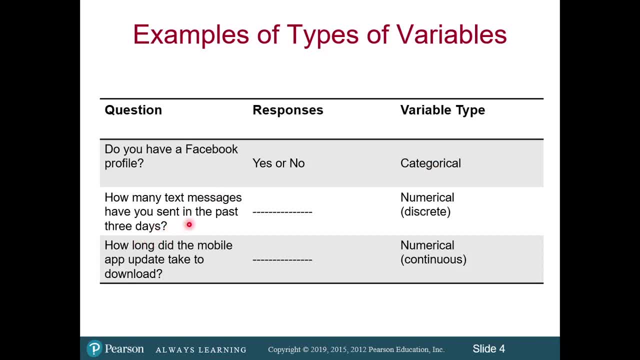 If question is: how many text messages have you sent in the past three days? In order to answer this question, what you need to do is to start counting Message number 1,, number 2, number 3, number 10,, number 20,, number 50, whatever. 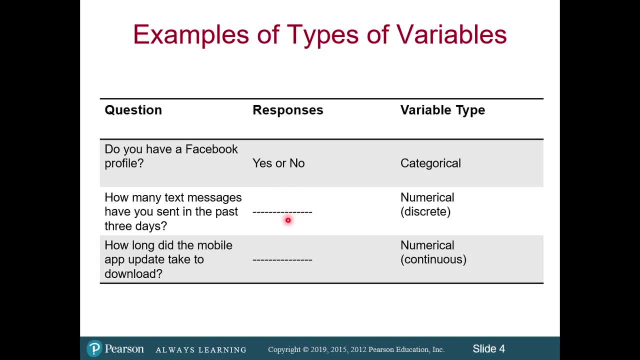 So after counting, you will be able to respond. I have sent 30 messages. Now this 30 is a numerical form, As this 30 arise from counting process. therefore it is a discrete variable. But if a question is, how long did the mobile app update take to download? 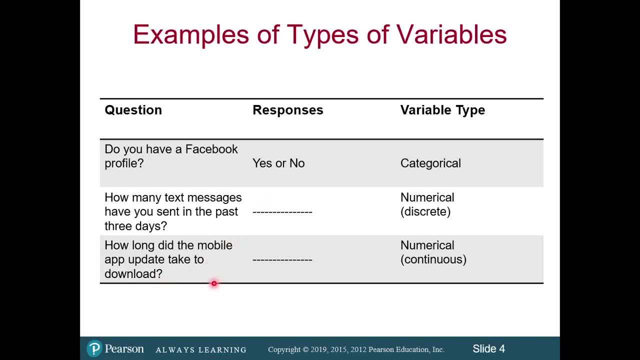 So you cannot count anything. You cannot answer yes or no. What you need to do, you have to have some measurement tools. You have to be able to observe how much time it takes to download. So what you need, You need a clock. 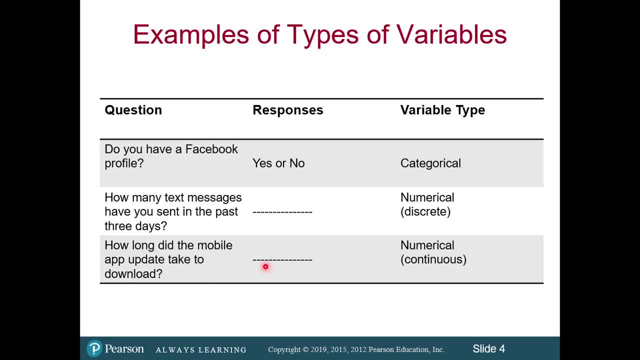 So this clock through which you can measure the time and then you can answer this question. So this is a numerical variable, but the form is continuous because it is coming from the measured process. So this is how we can easily understand the difference between categorical and non-categorical. 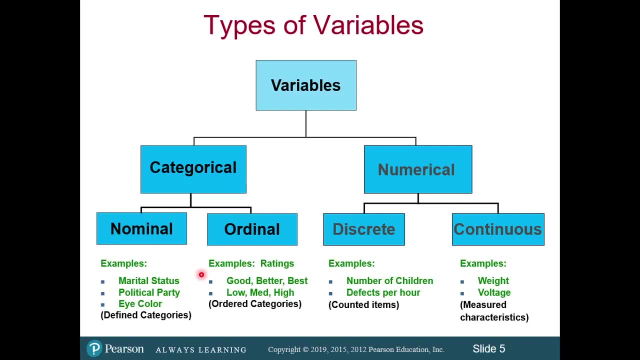 Now, under the categorical variables, there are further two forms: One is nominal and other is ordinal. Remember, nominal is very simple. It only defines categories. Just now I said yes or no, So that is the form of nominal. 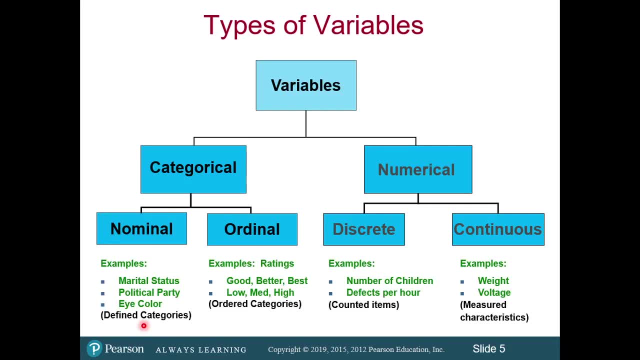 There is no order needed. Marital status: single, divorced, married, separated- Four categories, But can come here and there. There is no order, There is no order needed. But when it comes to the ordinal variable, there is the property of defined categories as well as ordered categories. 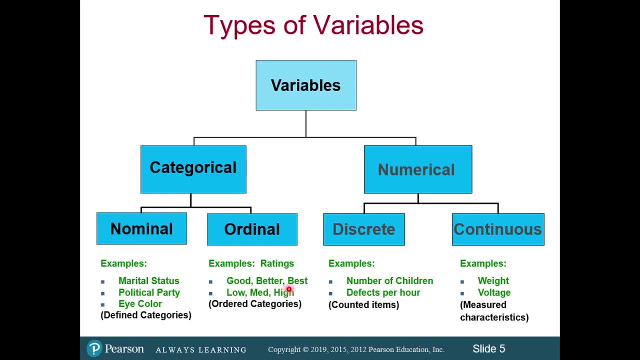 So you need to have some order: This better, good best. we cannot come like this. We always say good, better best. So three categories, and these are in order. Okay. So second, when it comes to the numerical variable, 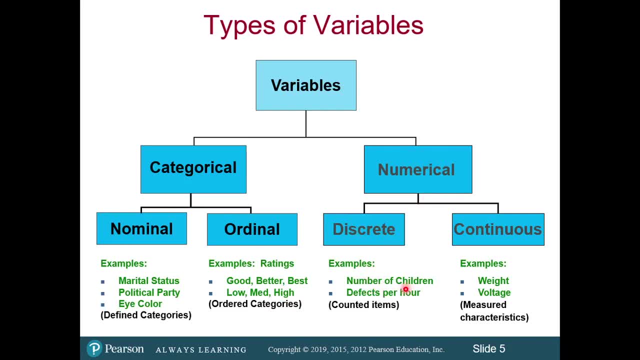 This is discrete, For example, number of children and your house. So you start counting 1,, 2,, 3.. Defects per hour: So you start counting how many defects per hour in a factory: 1,, 2,, 3,, 4,, 5,, 6,, 7,, 8,, 10.. 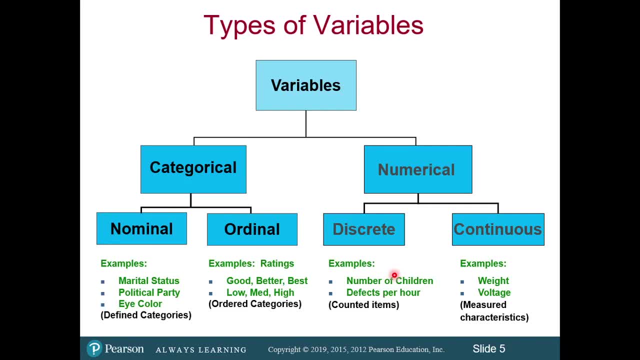 So 10 defects per hour in a factory, for example. So you started counting. Hence it is a discrete variable. But if somebody asks you, what is your weight? So you need a weight machine to weight your weight. 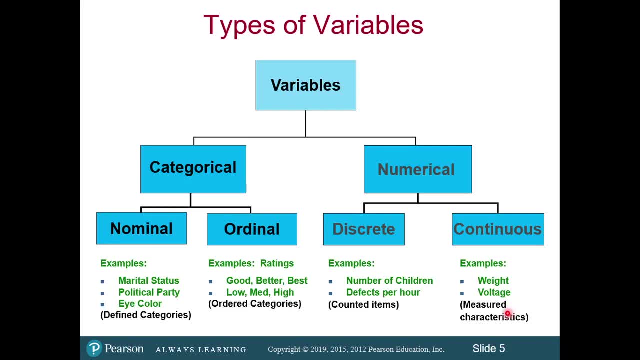 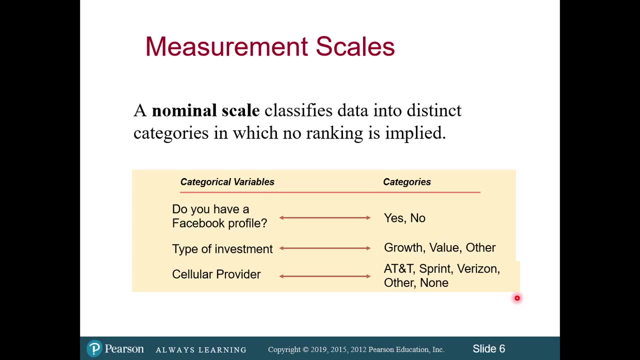 Right, That's why you have to have some measured characteristics. So this is the form of the continuous variable which comes through measurement. Now, when it comes to the measurement scales, there are four scales aligned with what we have just now discussed. 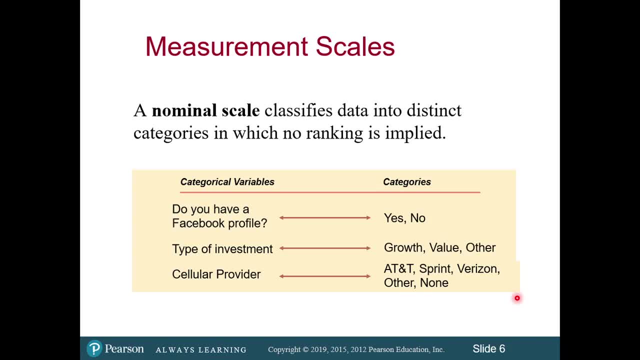 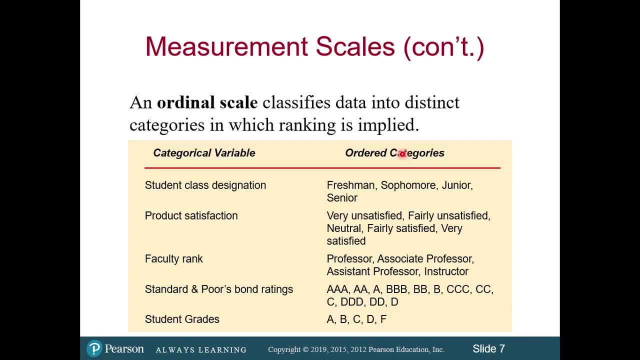 These four scales, as I said, one is nominal scale. Very simple. I already explained about what is. nominal scale. That classifies data into distinct categories in which no ranking is employed. Ordinal scale: it classifies data into distinct categories in which ranking is employed. 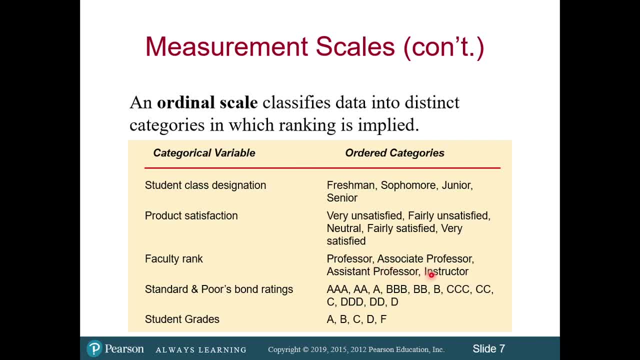 There is always a rank, For example instructor, assistant professor, associate professor and professor. There is no such thing like a person after graduation will join as a professor, Then he will be promoted. He will be promoted as assistant professor, then instructor, then associate professor. 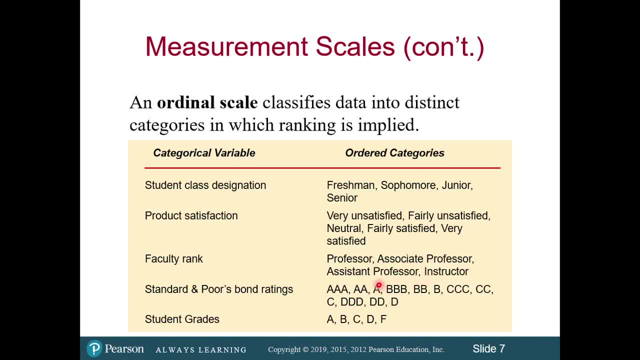 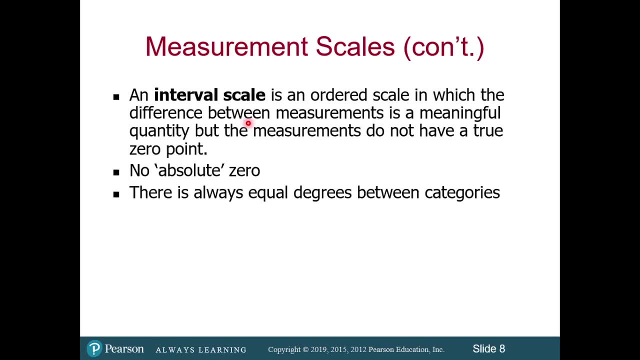 No, It always comes in order form: Instructor or lecturer, then assistant professor, then associate professor and then professor. So that's why this is the ordinal scale. When it comes to interval scale, it's very interesting to understand the difference. 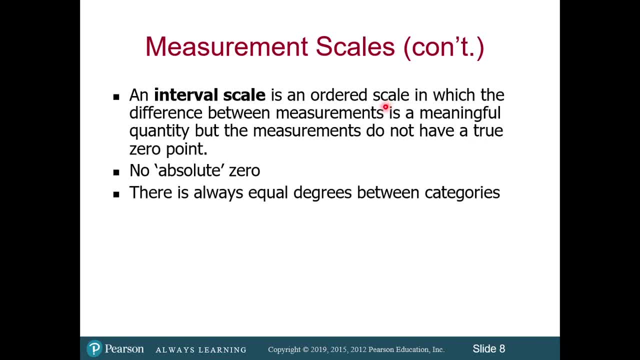 Interval scale is an ordered scale, You see. still, that is an ordered because it has the property of nominal and ordinal, But it has one additional property. It is an ordered scale in which the difference between measurement is a meaningful quantity, but the measurements do not have a true zero point. 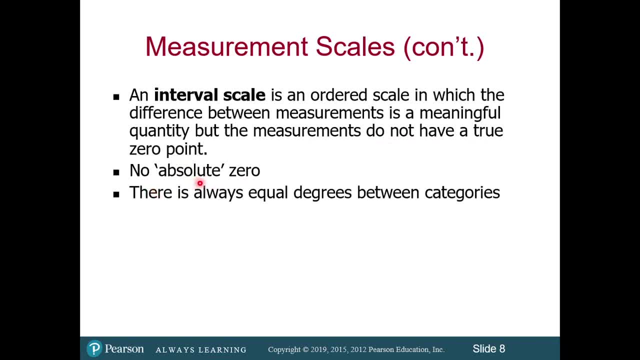 What does it mean? There is no absolute zero. There is no absolute zero in the data. There is always equal degrees between categories. For example, you are standing in a shopping mall. You want to observe the customers walking to a shopping mall. 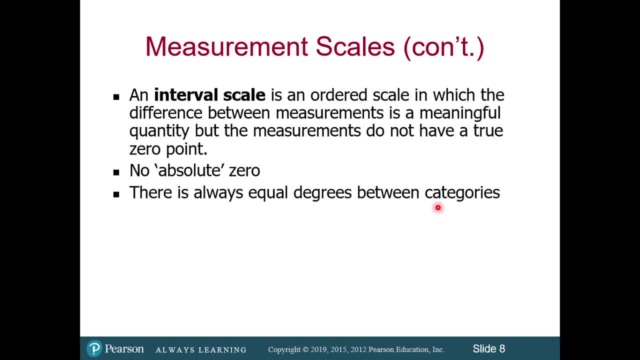 So customer number 1 came at 9 o'clock, The second one at 9.5.. Third is 9.10.. Fourth is 9.15.. So you can see there is an equal interval of 5 between the customer number 1 and number 2 and number 3 and number 4.. 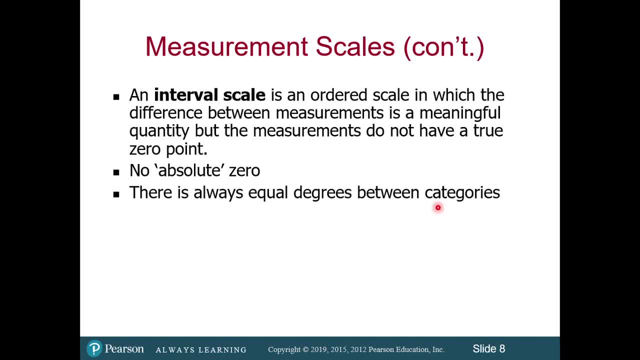 That is interval. But let's say if customer number 1 came at 9.. Second came at 9.2.. Third came at 9.7.. Fourth came at 9.15.. So there is no equal interval, So it is only an ordinal form. 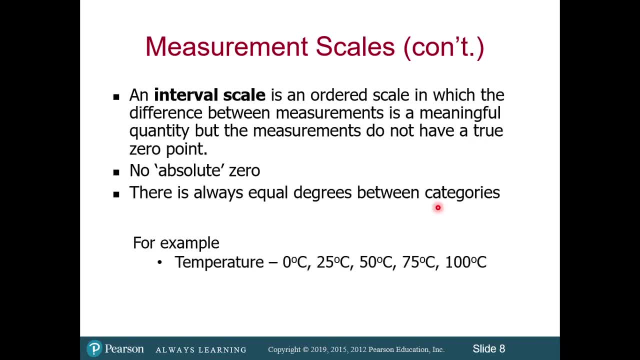 There is no equal interval. For example, temperature: Zero degrees centigrade, 25 degrees centigrade, 50,, 75 and 100 degrees centigrade. No absolute degree Zero. No absolute zero. Now you will be surprised to see. 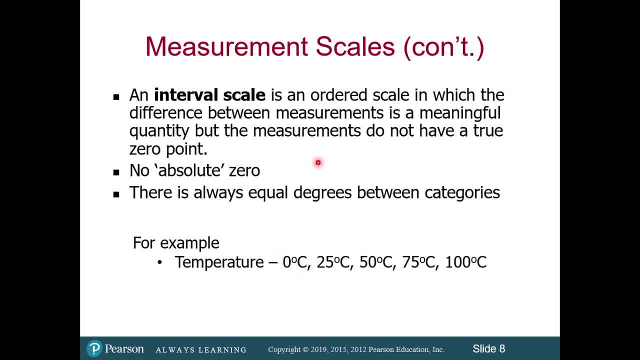 There is a zero, But what does it mean? Do not have a true zero point. The point here is true zero point. It means that this zero is not an absolute zero. When it comes to temperature, it can be zero degrees centigrade. 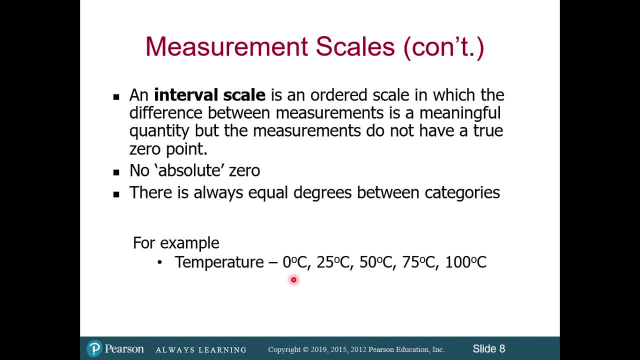 But it doesn't mean that there is no temperature. There is a temperature, But it's zero degrees centigrade. So this zero doesn't create any meaning. It is not an absolute zero. form Number two: There is an equal difference between categories. 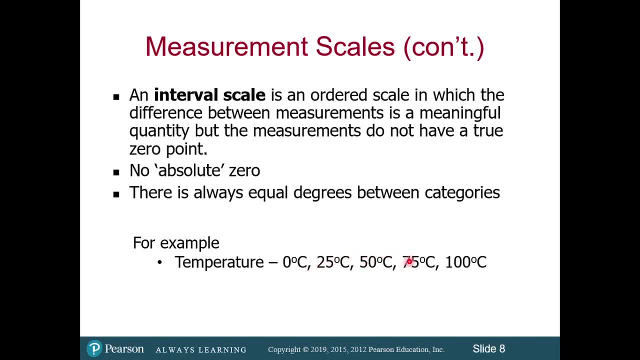 So zero to 25, 25 to 50, then 75, then 100. So there is a difference of equal categories, Difference of 25 degrees, For example, this 25 to 50. It doesn't mean that. 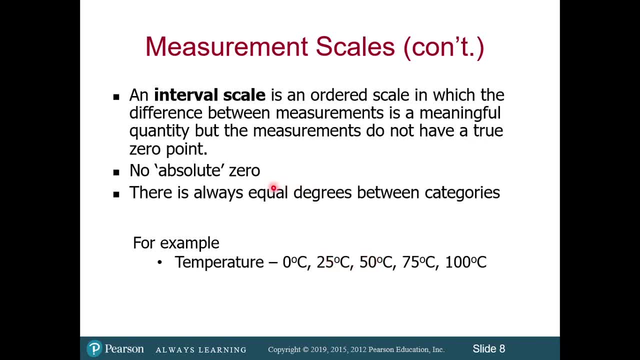 The 50 is the twice of 25. when it comes to the interval scale, It is the interval between two points And this, there is a zero, But that is not an absolute form, It's not a true zero. It is just giving us a property: that there is a temperature equal to zero. 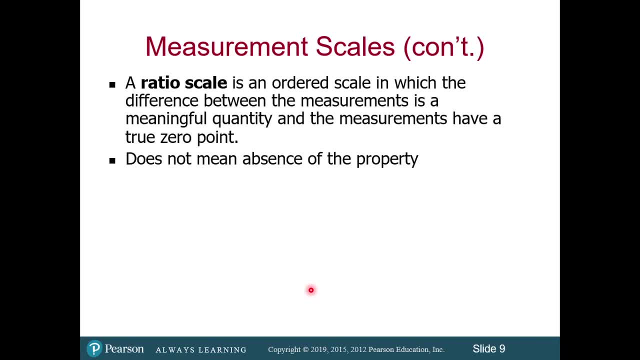 Now, when it comes to ratio scale, it is an order scale in which the difference between the measurement is a meaningful quantity- Same as just now we said about interval- And the measurements have a true zero point. This is the important point, Important difference between interval and ratio. 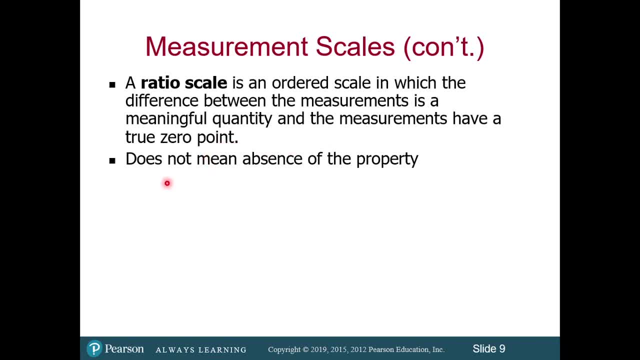 Measurement have a true zero point. It does not mean absence of the property. For example, weight Zero kilogram: 20 kilogram, 40 kilogram, 60 kilogram. Now you see this zero kilogram. It means there is no weight. 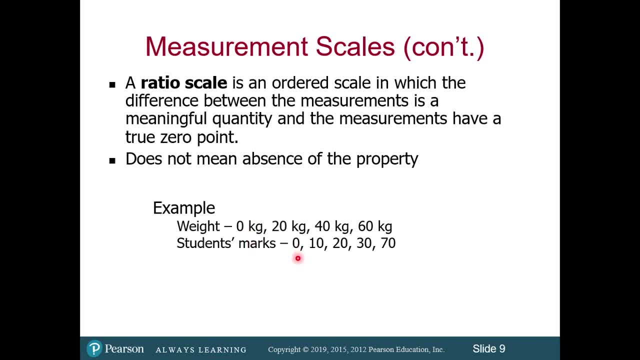 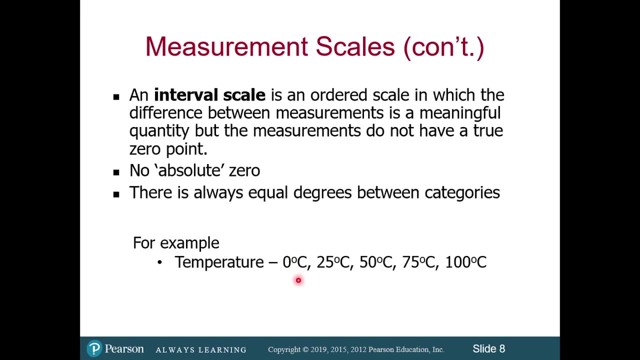 Zero marks. There are no marks. So now, that is a true zero. It is not an absolute form, That is a true zero. When there is a zero, it means nothing, But here, when it is zero, it doesn't mean nothing. 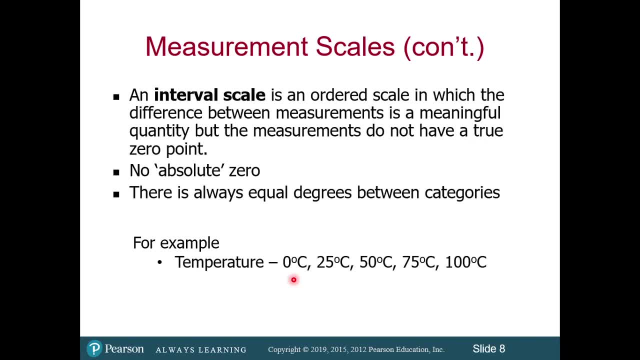 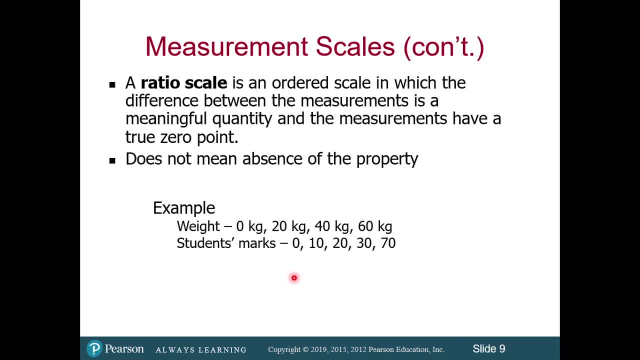 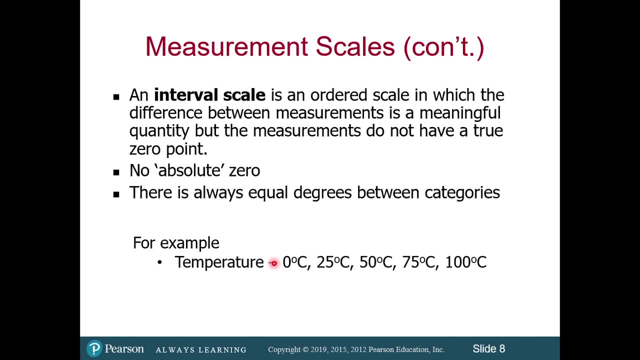 There is a temperature. Its category is zero, degree Its degree. So that is how we differentiate between interval and ratio scale. So this zero create a meaning Does not mean absence of property. Here zero property is available, But here the property is absent. 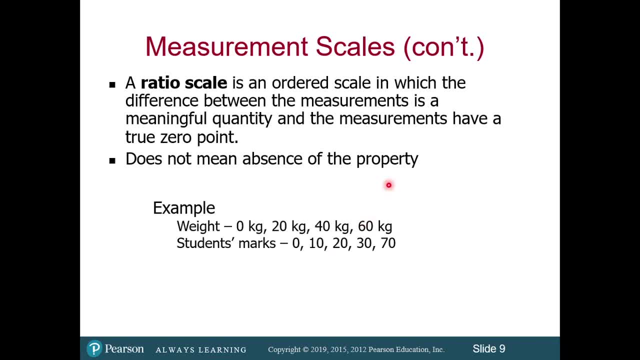 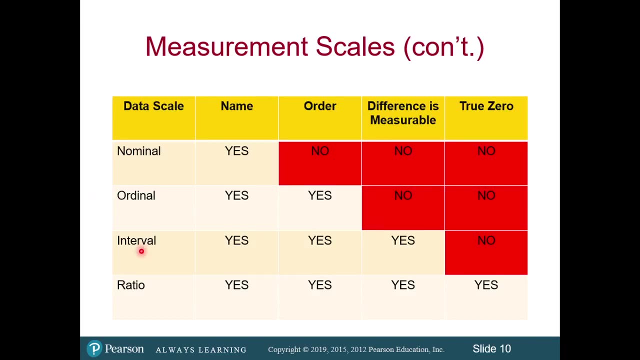 So for ratio, we always need a scale. For ratio, we always need a scale That we use to measure its properties. So, concluding, when we plot in a way, nominal scale, ordinal interval and ratio scale, And we want to give them in this order. 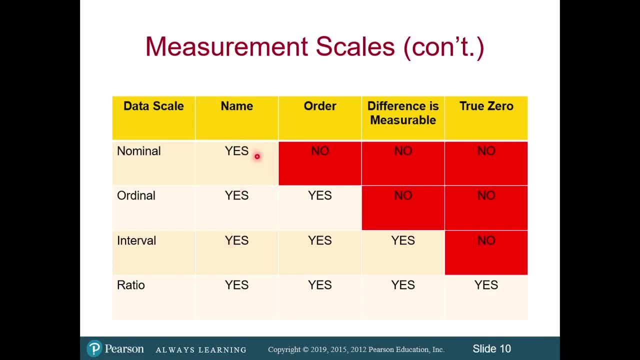 So when it comes to the name of categories, defining categories, So all have the same properties? Yes, we have to define categories. We need to give order. For nominal, no need, But for ordinal interval and ratio. yes, Difference is measurable. 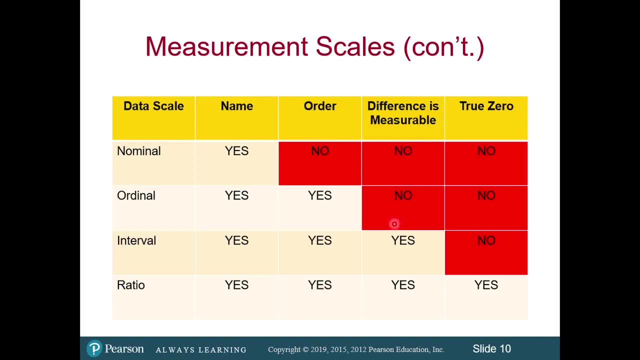 When it comes to the difference between two data points, In nominal and ordinal difference is not measurable, But in interval and ratio difference between two data points is measurable. And finally, true zero: For nominal, ordinal and interval, there is no true zero. 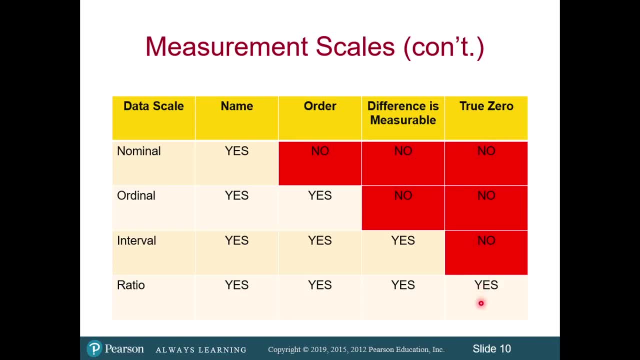 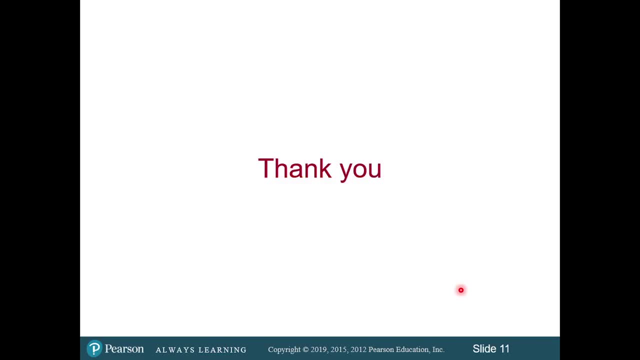 But in ratio, zero means real zero, Zero means real zero. So this is how we understand the classification of variables and the types of scales. Thank you, 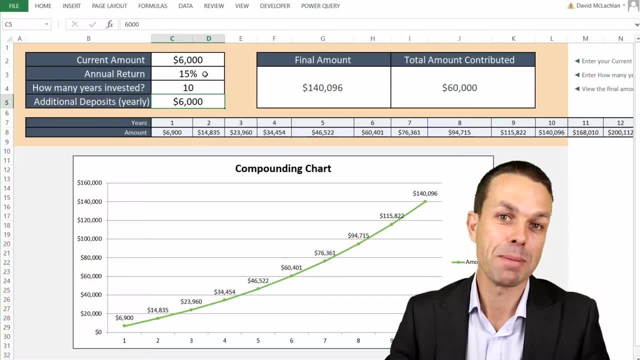 Hi everyone. I make PowerPoint and Excel templates to help people get ahead in their career and get the most out of their business and their organisation. This one in particular is a compounding chart. But what is compounding? Well, it's been described as the eighth wonder. 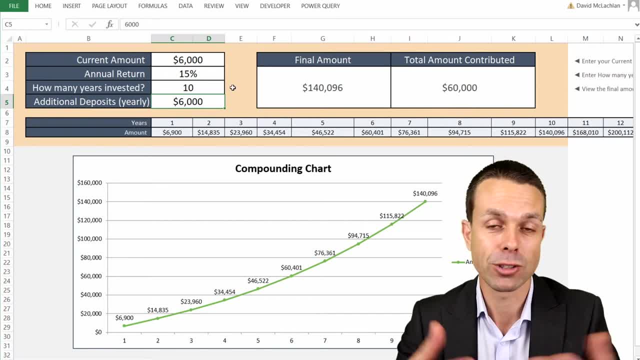 of the world where we have an initial amount that we invest, maybe in stocks or in real estate. We get the return on that money, but we reinvest that money And so eventually this reinvestment amount starts small but we're constantly reinvesting, reinvesting. 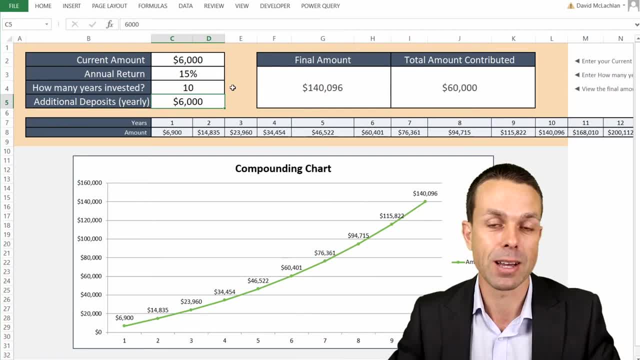 and it's like a snowball rolling down a hill. So it eventually ends up as a large amount, with the returns becoming larger and larger and larger, based on the percentage of the amount that you have. So let's see an example of this. Let's say we managed to save $6,000. 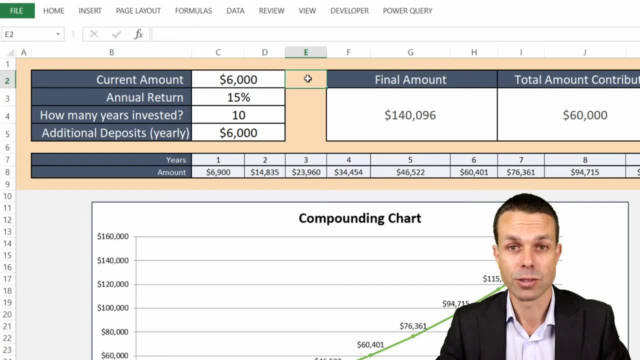 this year, That's say $500 a month. Hopefully some people might be able to do that. You might be able to do more. for example, And let's say we got 15% a year, putting that into the stock market, And again it could be. 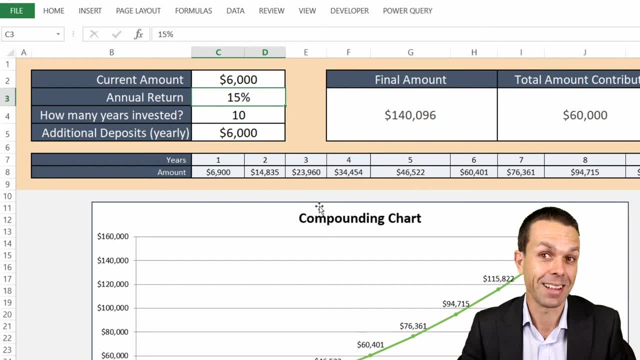 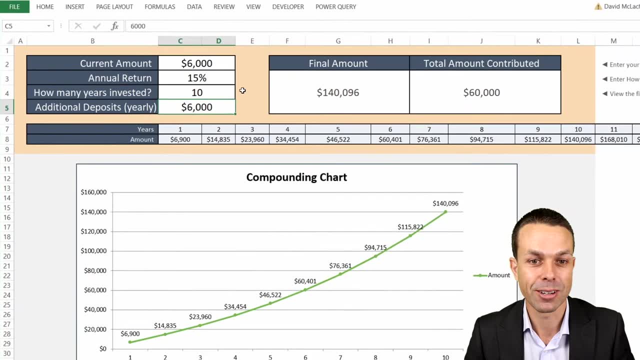 more or it could be less, but we can change this on our compounding chart, and that's the beauty of it. And let's say we invest it for 10 years And let's say we're adding another $500 a month, so $6,000 a year, roughly every year. Well, over 10 years we can see. 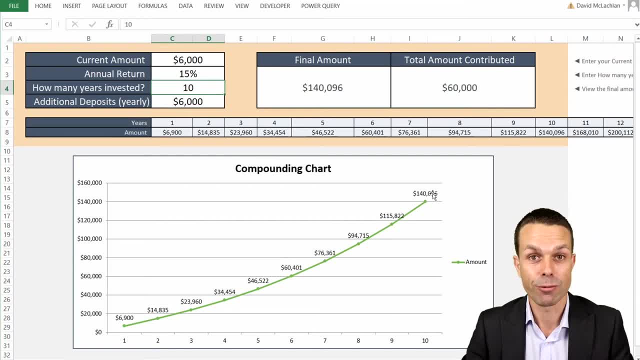 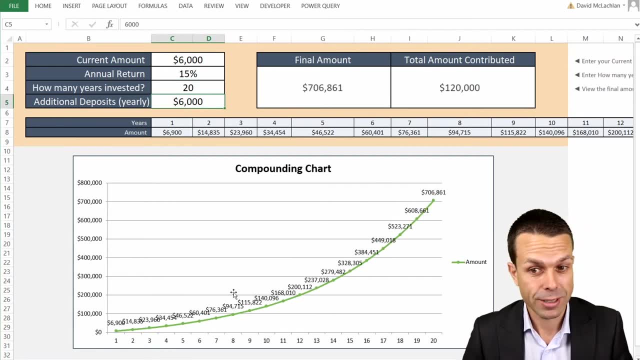 that it will have grown to $140,000 in total. But what if we started doing that and kept doing that for 20 years in total? Well, all of a sudden it's now around $700,000, just from $500 a month. 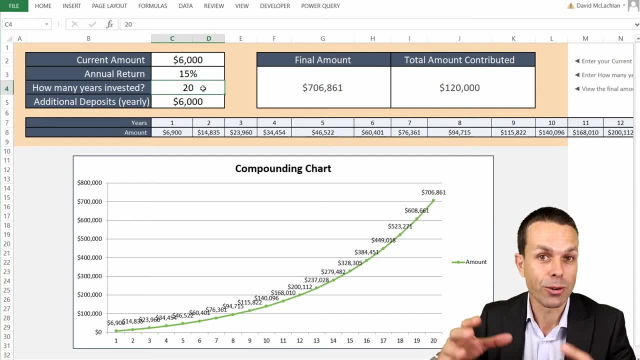 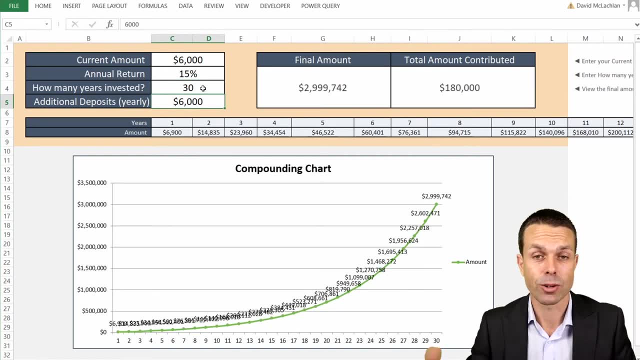 Now the time factor is really important because that snowball is getting bigger and bigger and bigger And those returns reinvested are getting bigger again. So let's say we did this for 30 years in total, so across our working life, for example. Now, all of a sudden,